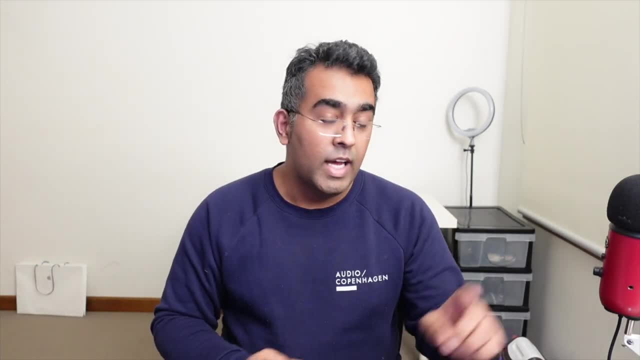 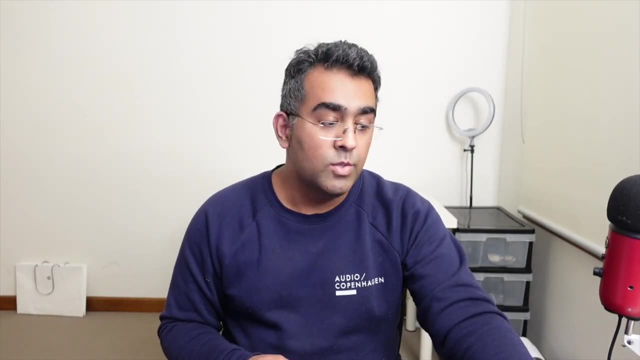 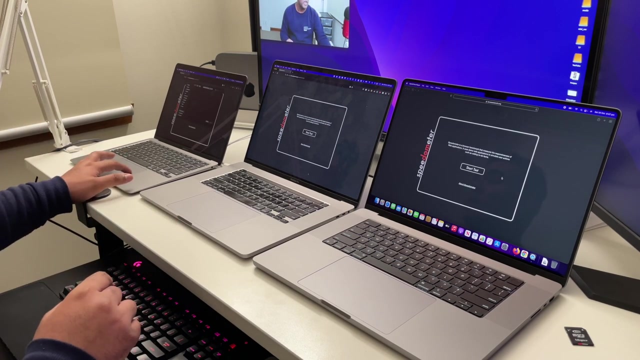 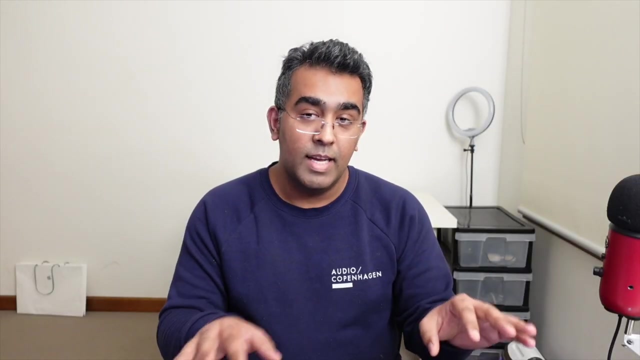 And 16 GB on the M1 Pro, And also I have this MacBook Air with. it's basically a base model. So what we're going to do is we are going to use three browsers: Safari, Chrome and Firefox. First test we're going to do is going to be on Safari on all three computers and see what scores we get. Next I'm going to run the same test on Chrome and let's see what results we get, and then on the Firefox. 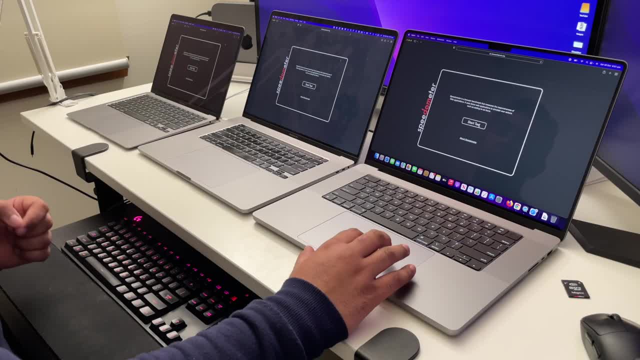 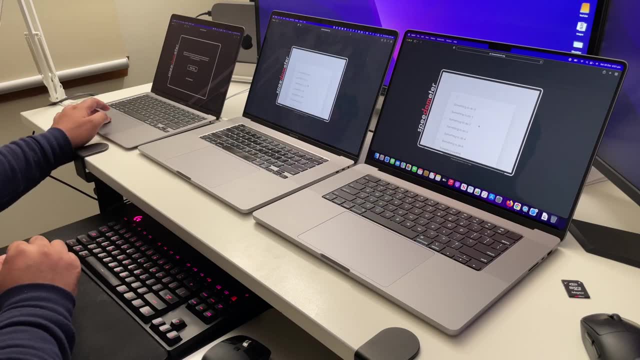 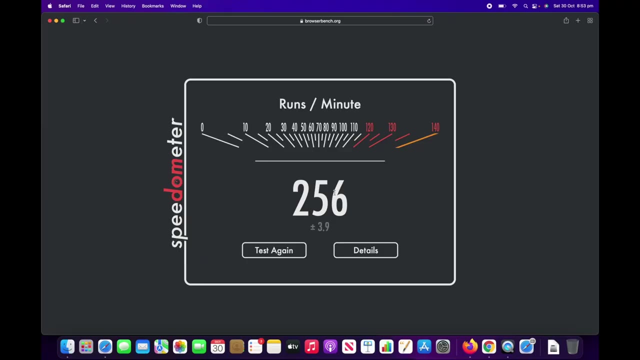 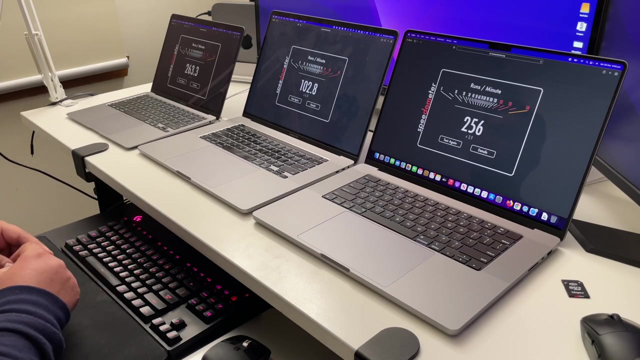 Okay, so let's start our test on M1 Pro, on Safari browser, on Intel i7 and then on MacBook Air. Okay, so we have the results. on M1 Pro 16 inch, We have 256. Intel 16 inch, We got 102, and we also have results on MacBook Air, which is 263.3.. And by looking at these results, guess what? 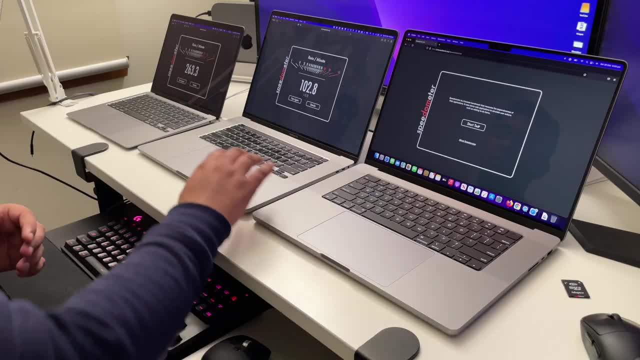 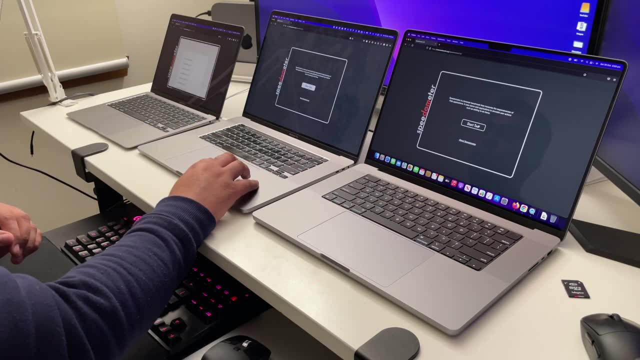 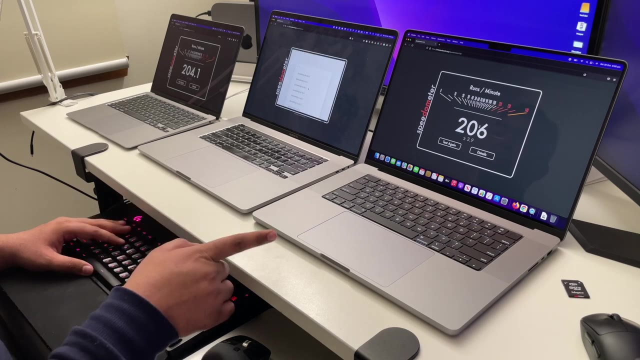 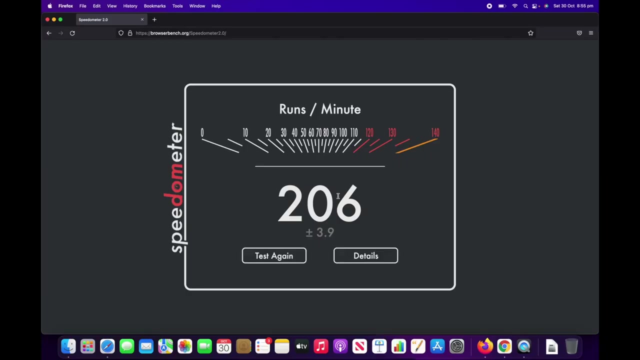 We actually won. Now let's go and run the next test, which is going to be on Firefox on all three computers. First let's do the Firefox on MacBook Air, Firefox on Intel and Firefox on M1 Pro and one pro finish. So we got 206 on Firefox and one pro actually beat MacBook Air by two points And the difference is actually quite significant compared to Intel. 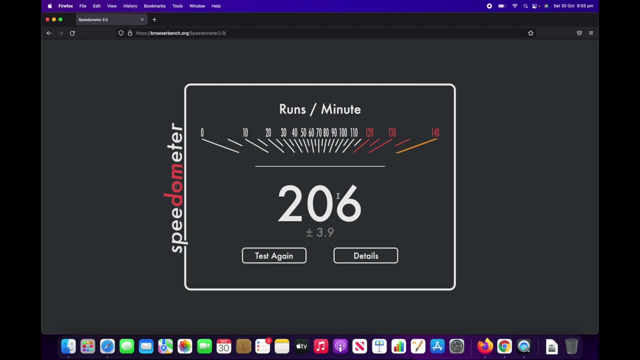 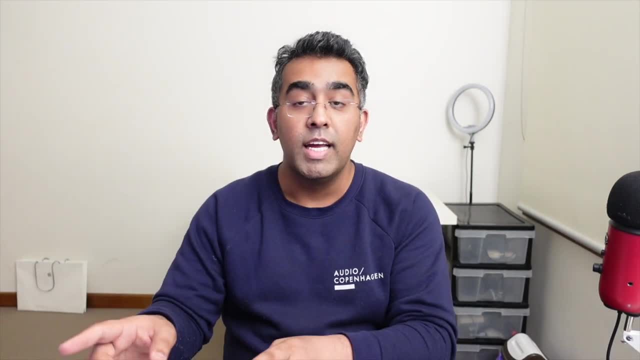 Intel and Apple silicon to get 80 points on Intel MacBook Pro 16 inch. The last test we're going to run is going to be Google Chrome, And I'm running a native Google Chrome on these two MacBooks, which are Apple silicon ones to run on Chrome. 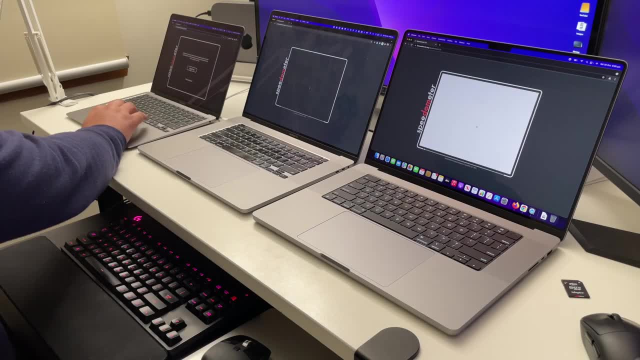 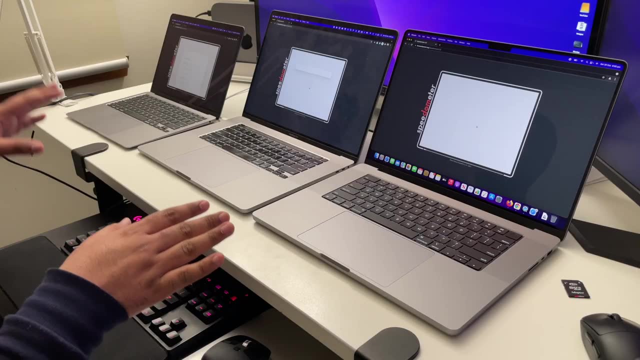 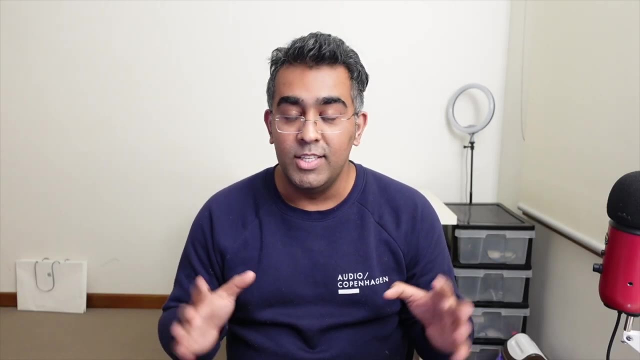 And let's run on the Chrome on Intel as well And on MacBook Air. let's start the test on Chrome as well. So this is going to be very interesting, because if MacBook Air beats this M1 Pro pro, i'll be very, very surprised. and yeah, you can see for yourself how these computers are performing.